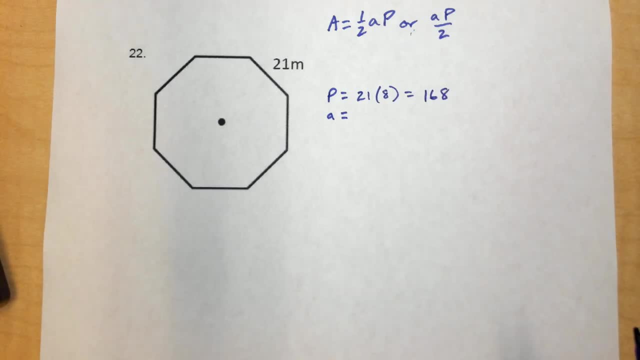 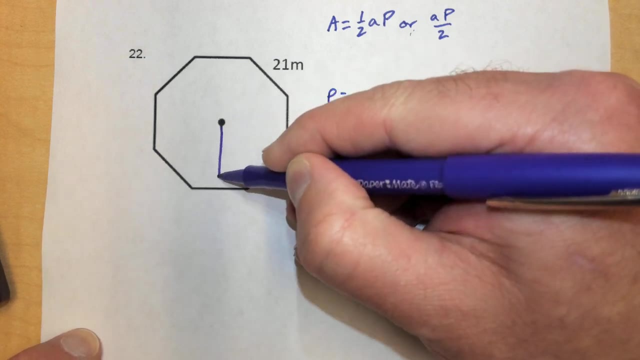 The apothem, though that's kind of where this gets a little bit tricky, because we're going to have to solve for that. So keep in mind, the apothem is the distance from the center of the shape to the side, And it's going to have to meet at a perpendicular And that's really important. 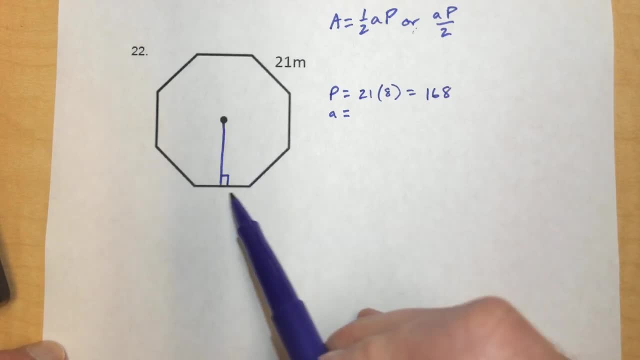 because that perpendicular allows us to solve for the distance from the center of the shape to the side And it allows us to use some properties of right triangles, which we're going to do here in a minute. But since we don't have that, this gets a little bit tricky because we're going to have to 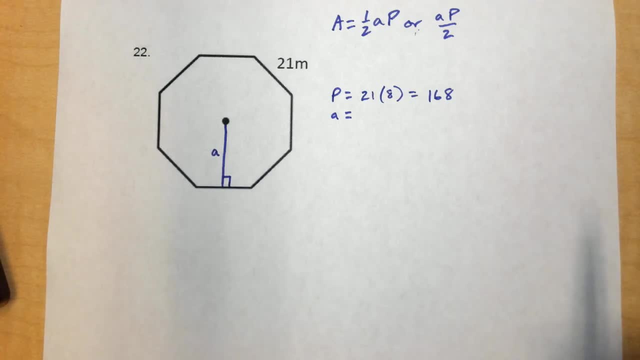 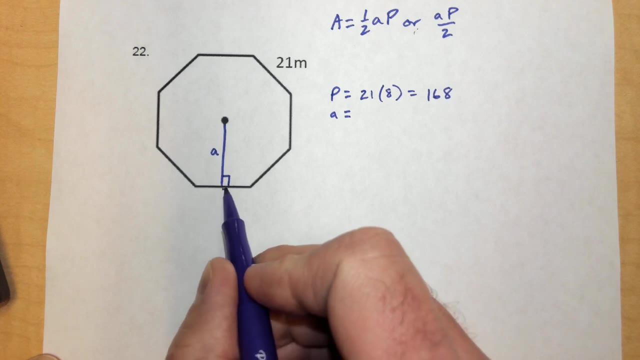 use some trigonometry here. We don't have enough information really to solve this. One thing you need to know, though: because we are going to be using a triangle, we need to know what this distance is here, And keep in mind that apothem, when it comes from the center down to the side of 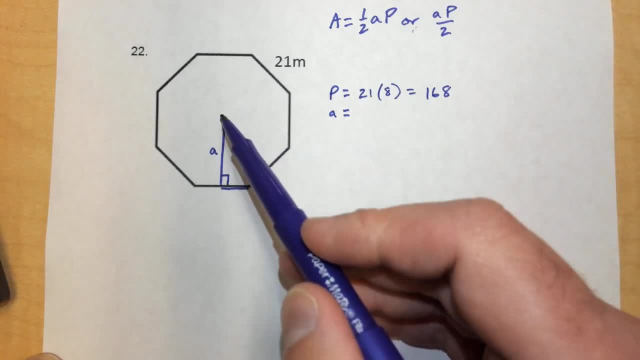 the shape cuts this side in half. Okay, And it's going to end up cutting these angles And so we're going to have to- uh, but it cuts that side in half. So we need to know that. this side right here, 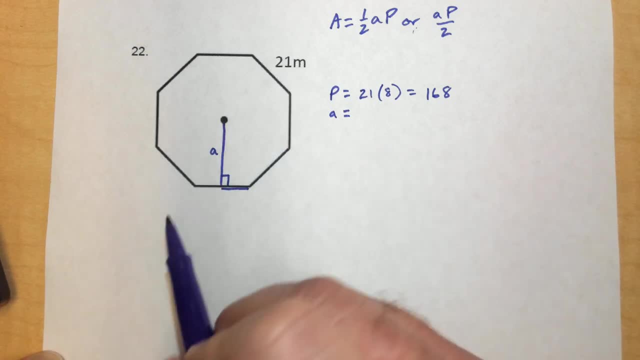 of the right triangle we're about to create is going to be half of the 21.. If this whole thing is 21,, then that part from the apothem over to the uh the corner is going to be half of the 21,. 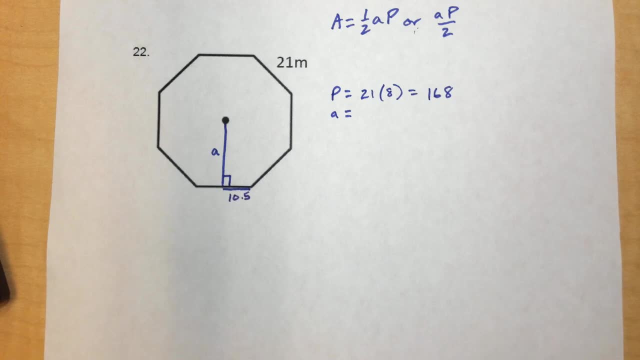 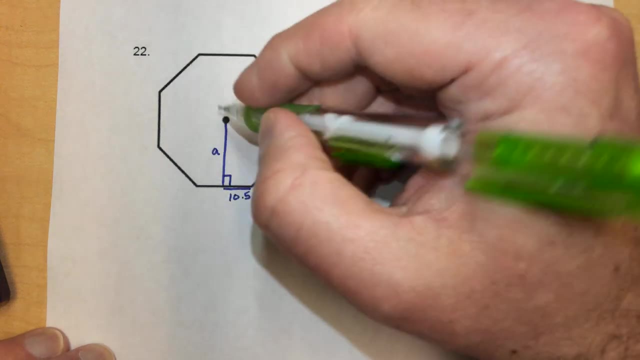 which is 10.5.. So we're going to be using that here in just a second, Uh, but first we need to find some, some angles here, because we don't have enough information. If we had, if we had this radius or something like that, we wouldn't have enough information to solve this. So we're going. 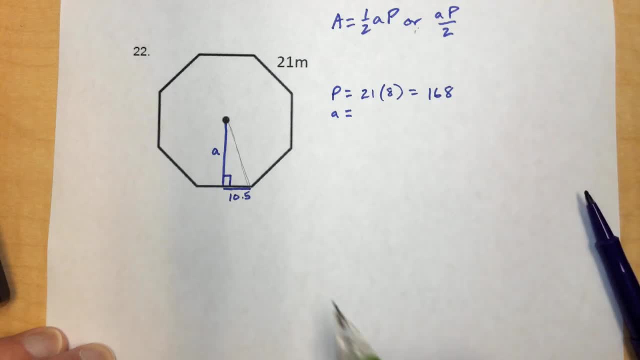 to have to figure out an angle, either the top angle or the bottom angle, And then we're going to use some trigonometry in our right triangle. So I'm going to show you how to do both: uh, finding the angle for the top and finding the angle of the side. here Again, you are only going 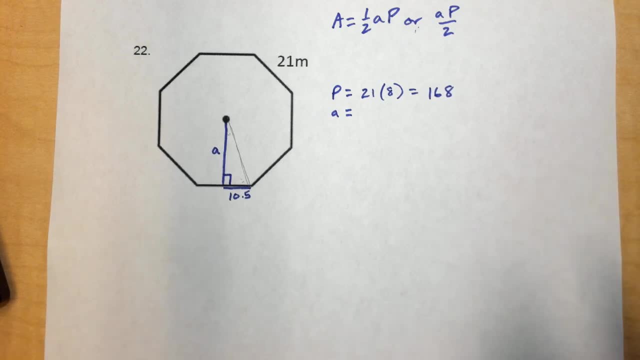 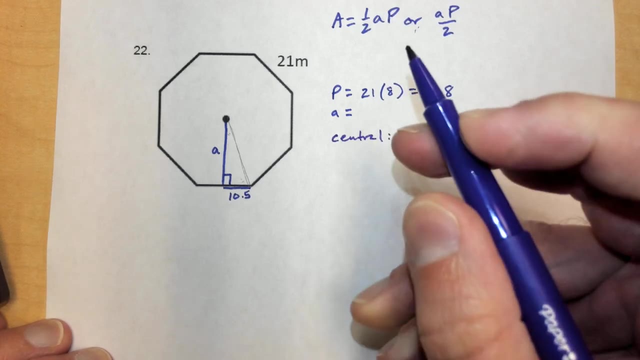 to pick out uh one uh method to use, because it doesn't really matter. You're going to get the same thing. So we're going to have to figure out an angle here, And then we're going to have to find the central angle, And I'm going to show you how to do that. Or we're going to find uh one. 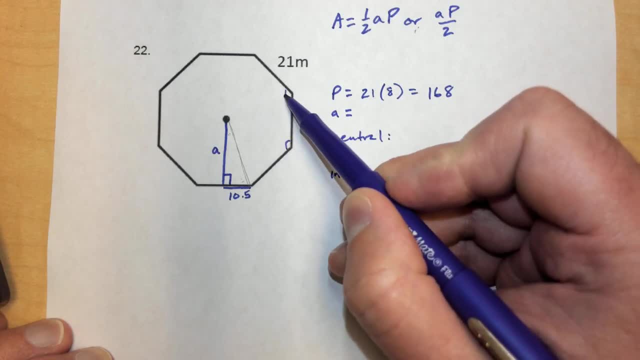 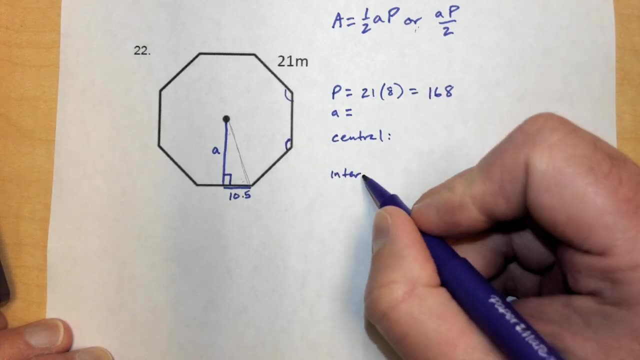 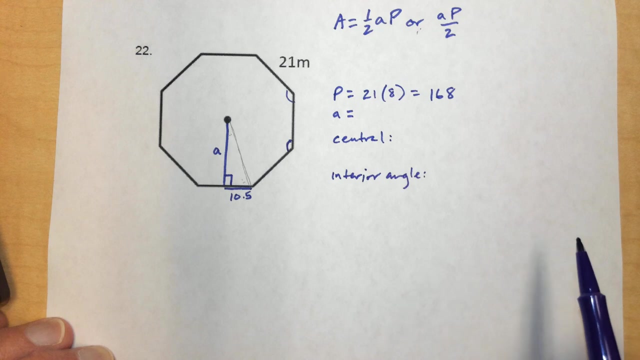 of the interior angles. which are these right here? Okay, Central angles would be at the center of the circle. Uh, the other, uh, interior angles would be here on the side. So we're going to find, uh, both. again, you choose one that you want. Okay, So to find the central angle. 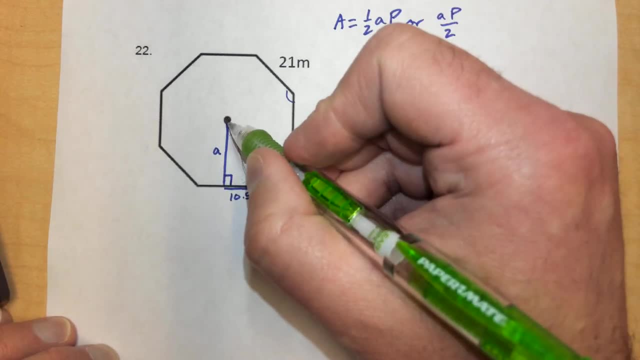 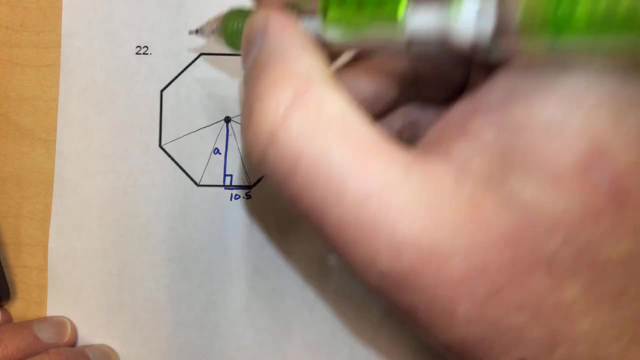 and I think some of you might find this a little bit uh, easier, because we just covered circles not too long ago And if you were- if you'll keep in mind- if we were to split that circle up, it kind of works the same way as we're doing right here: We're splitting this shape. 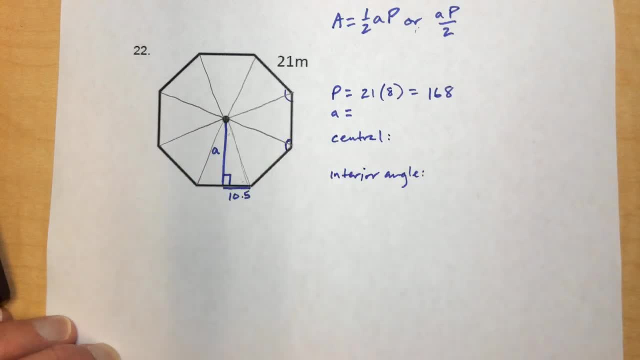 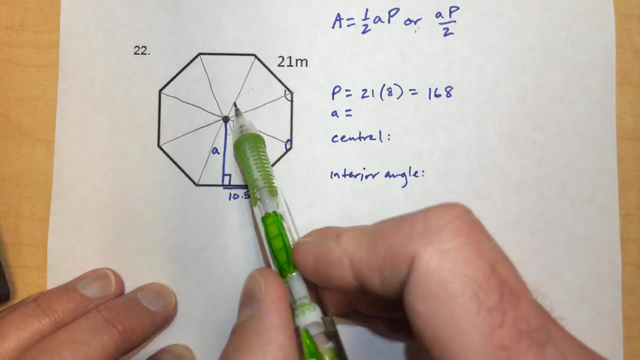 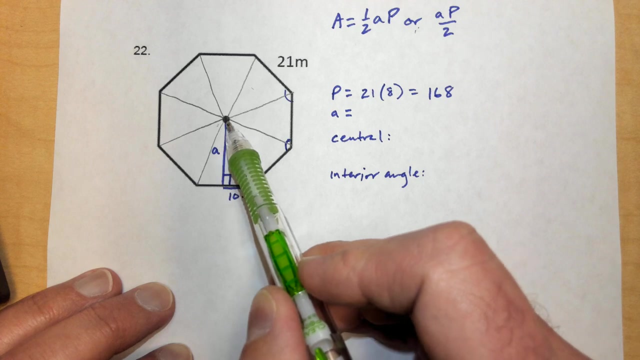 up into triangles. Okay, If we can split that up into triangles, then the number of triangles is the same as the number of sides, And so what happens here in the center, though, is: you've got the, the apex, or the top part of this triangle. here is, uh is, a central angle, since it's attached. 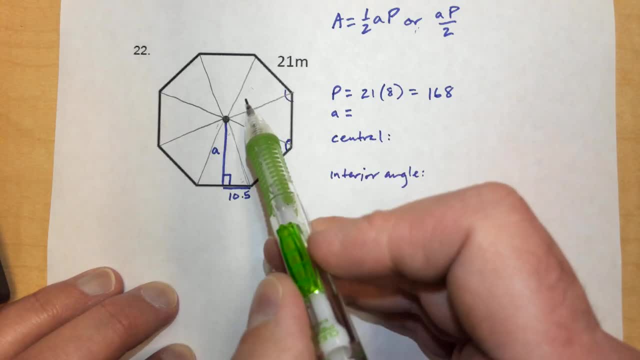 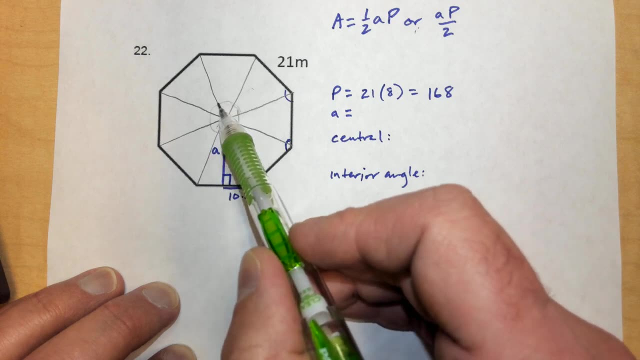 to the center of the shape. That's a central angle And if you remember from our circles lessons, all of these central angles here, just like they do in a circle, have to add up to 360 degrees. So, because all of these will be the same, because all of these 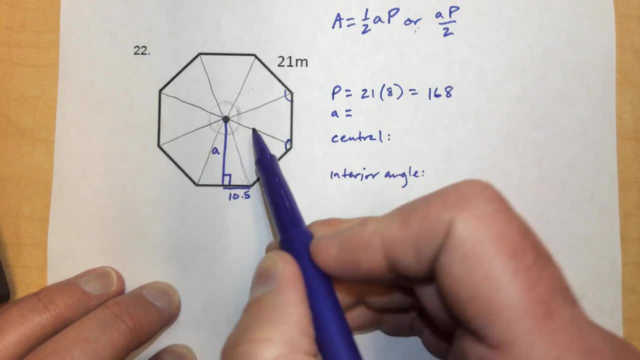 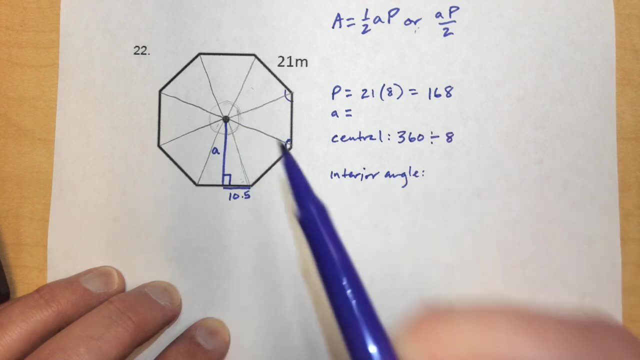 triangles are the same. we can just take the 360 degrees here in the center and we can divide by the number of angles that we have. And since there are eight of these uh triangles, there's eight of those angles. We divide 360 divided by eight and that'll give us a central angle. So we're 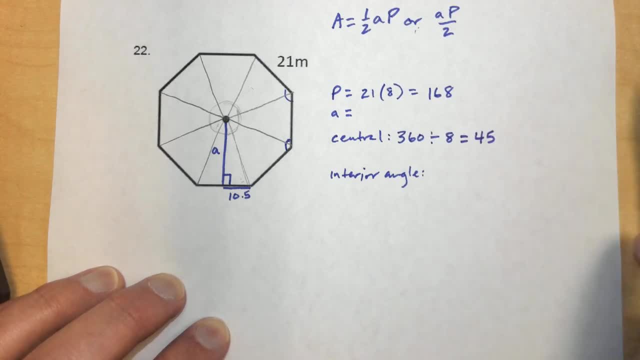 going to have a central angle of 45 degrees Now in our right triangle, though here, if we draw that radius in, keep in mind this apothem is going to split this angle into halves, So this angle here is 45 degrees. Then the the top part of our right triangle then has to be half of the 45 degrees. 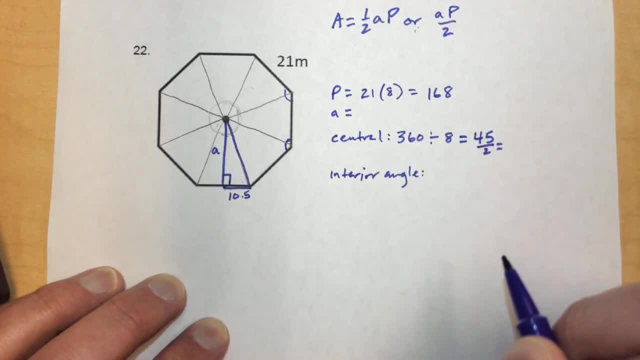 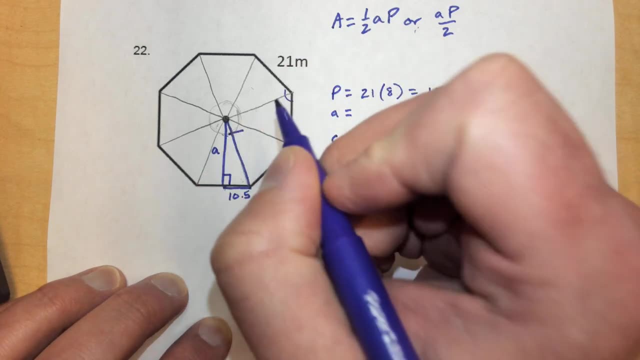 So if we do the 45 degrees divided by two, then we have a central angle up top That would be 22.5. degrees. So that angle up here is 22.5 degrees And then we can use that in trigonometry and we'll. 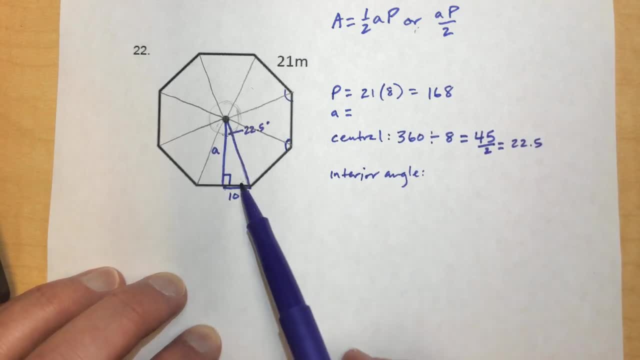 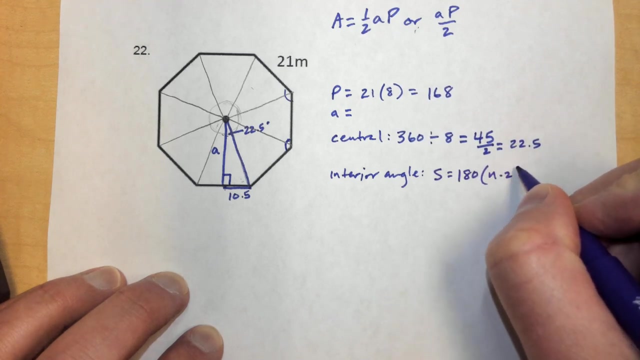 show you how to do that here in just a second. Uh, we could also find this angle using a different formula. Um, if you'll remember, from uh, unit seven, I believe it was, you can find the sum of all interior angles by using the formula 180 times the number of sides minus two. And because they're all 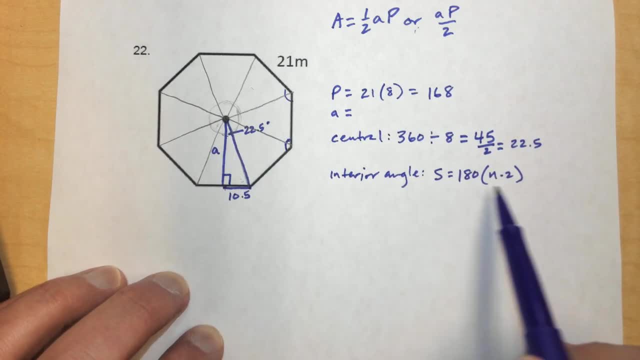 the same. we're going to divide by how many there are to figure out how many sides there are. So we're going to figure out each one. Let's figure out what the total of all these angles will be by plugging our number of sides into our formula. So our the total of all interior angles are going to. 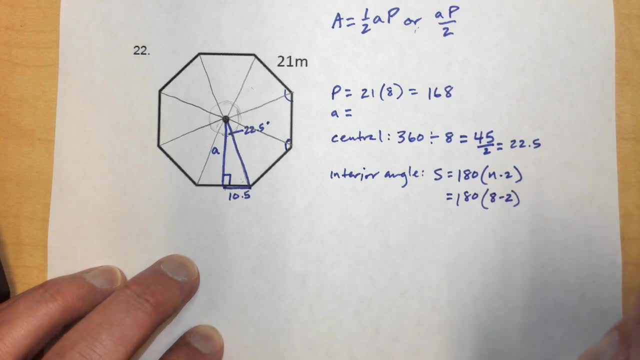 be 180 times our number of sides, which is eight minus two. We'll solve the parentheses first. That's 180 times six, which is 1,080 degrees. So all of these uh interior angles here, all of these big. 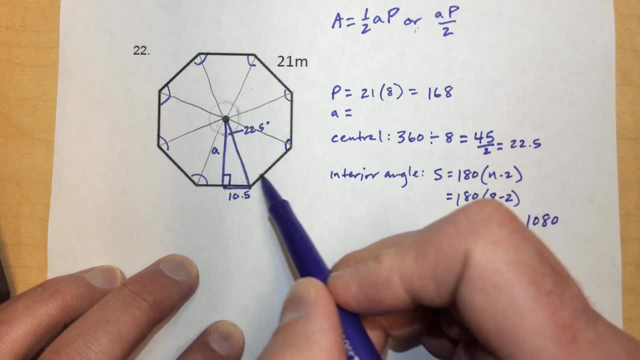 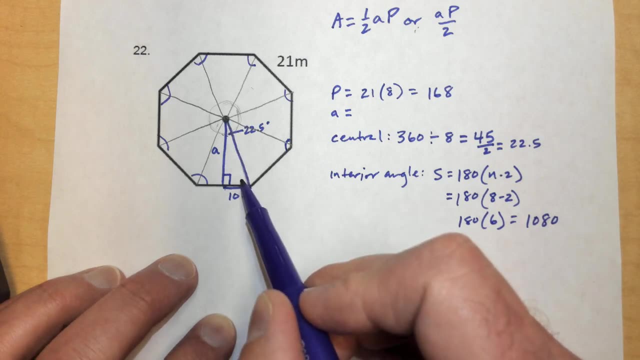 angles, uh, have to add up to a third of the interior angles. So we're going to do that here. So if we just take our angle and divide it by the width, we add up to a third of the interior angles. So we're going to divide by the width, we add up to a third of the interior angles, So that is 1,080. 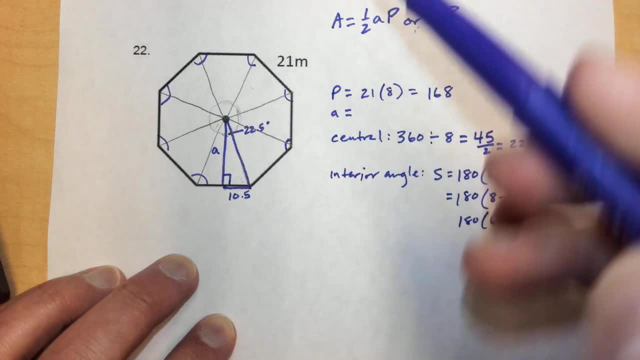 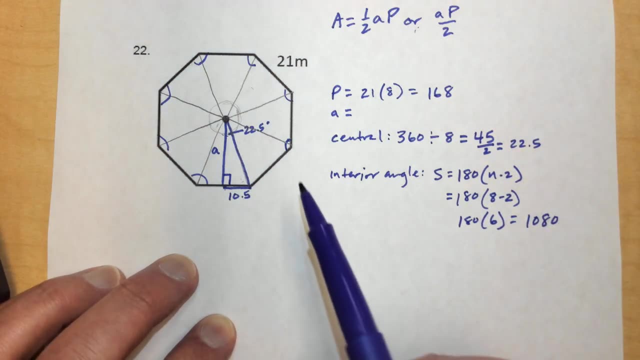 degrees and including this one right here, But because we only want this part of our angle. in our right triangle, if you'll notice, this radius that's coming down from the center to the corner, that radius is also going to split this angle in half. And if this angle here, if we can, 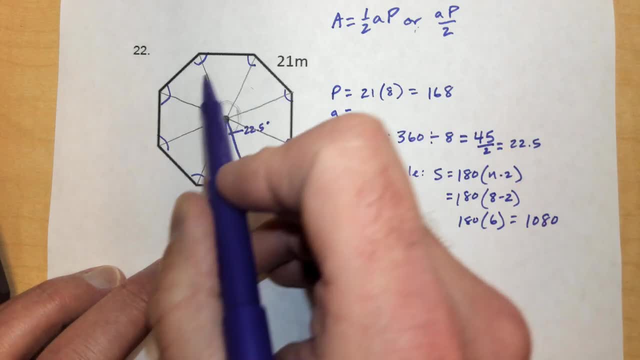 figure out what that angle is. we just divide that in half and figure- uh, figure out what we have for our triangle. And because there are eight angles here that are all going to be the same, we divide our total of 1,080 divided by eight. 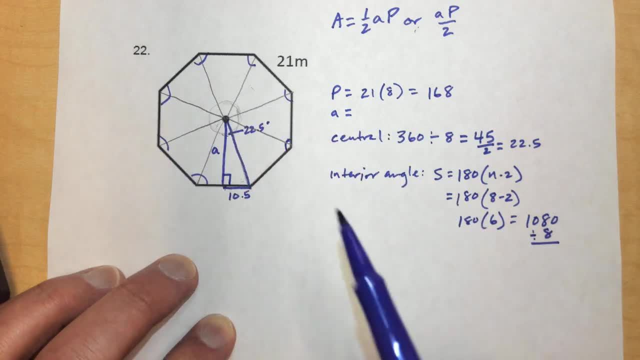 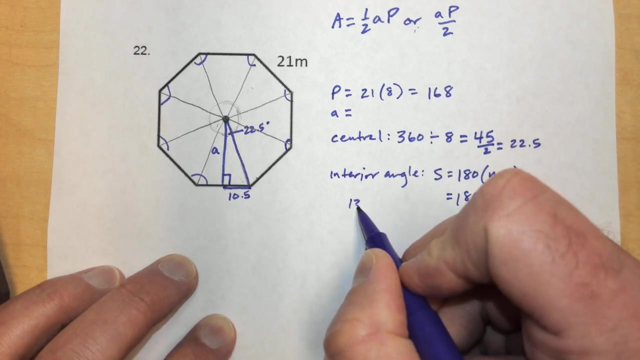 So each one of these big angles on the interior have to be 135 degrees, And since we only want half for our triangle, since this whole angle is 135 degrees, we're going to split that in half to get the angle here. So 135 divided by 2 is 67.5.. 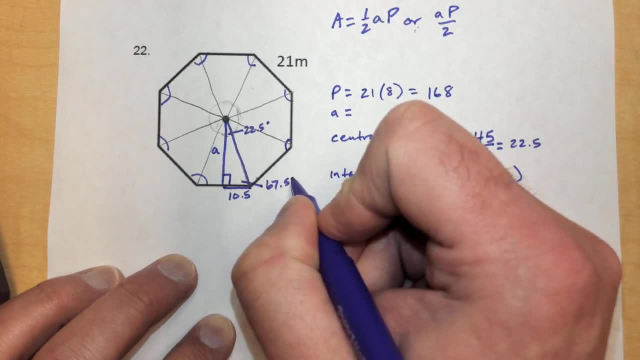 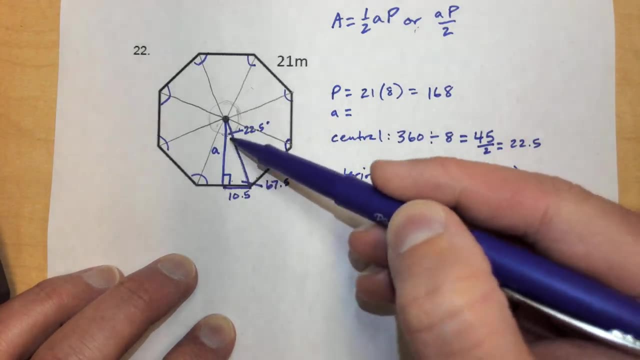 So this angle here is 67.5 degrees. Now we figured out both of them. It makes sense. These two have to add up to 90, because we have a 90 degree there. All of these add up to 180.. So we've done our math right. 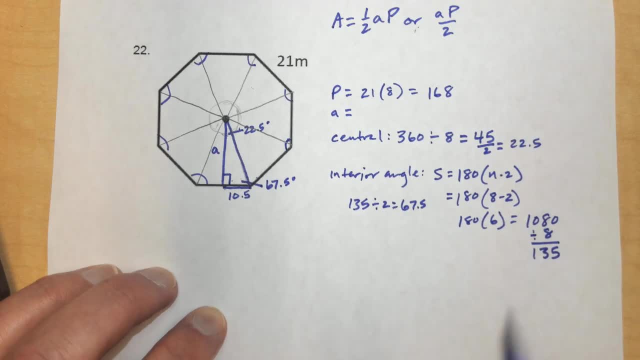 But now we're just going to pick one of these. I'm going to do both again for you. You are going to pick one, whichever method you prefer, whether you do the central angle or not, whether you do the bottom right-hand angle over here or not, 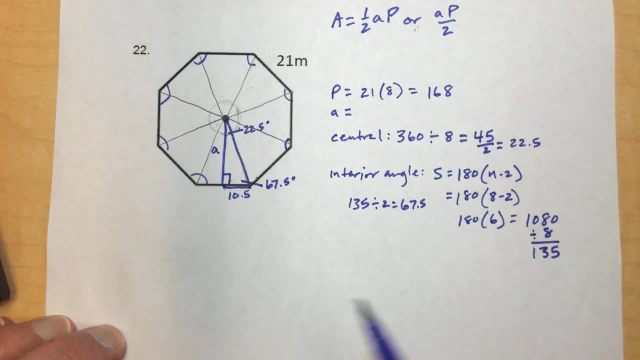 It's up to you, You can choose either one. But now that we have an angle, we can use some trigonometry to figure this out. Remember, trigonometry is either sine, cosine or tangent, And since sine and cosine both use the hypotenuse of a right triangle, which is our radius here, 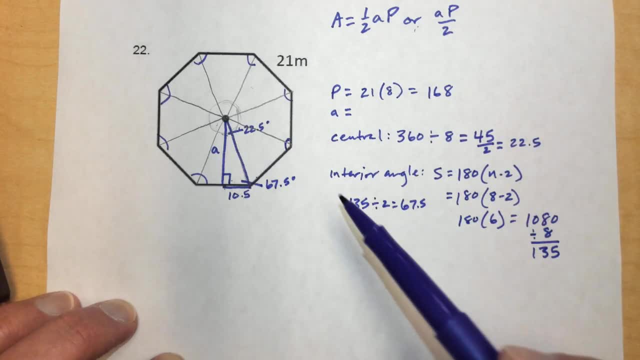 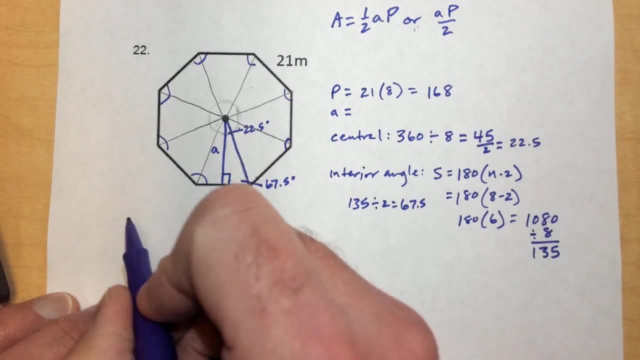 we don't really care about using either one of those, because we don't need the radius. All we're concerned with is the legs of our triangle, if you will, because that apothem is one of the legs of our triangle. So we're going to use the tangent function. 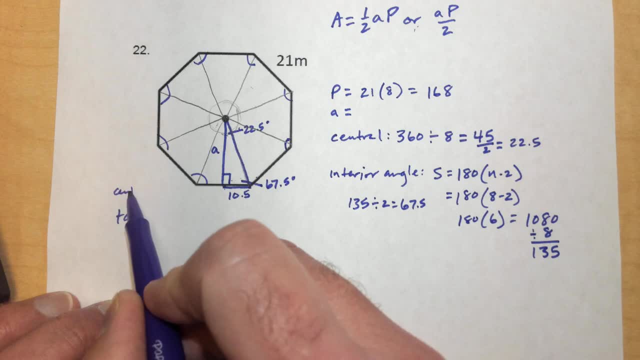 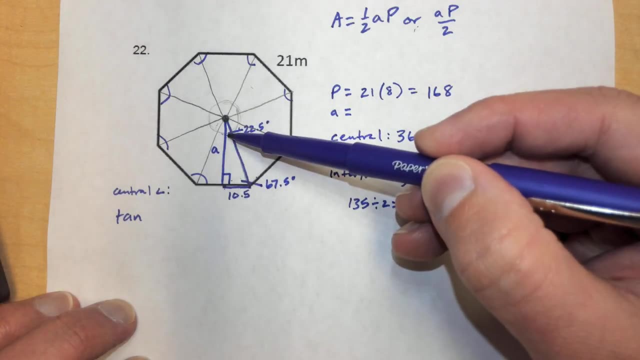 And so if we're using the central angle, we're using the central angle here on this one. We'll start there because we can use the 22.5.. 22.5 is the tangent function. It's still going to be a tangent function, okay. 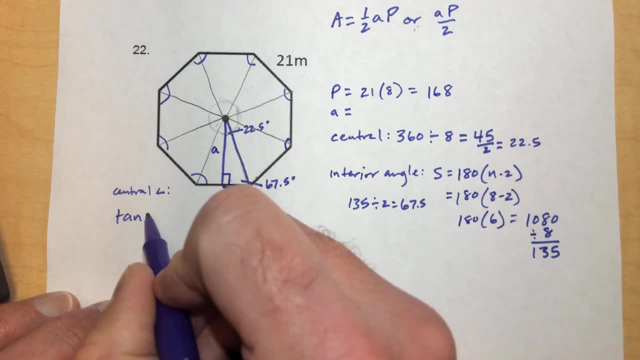 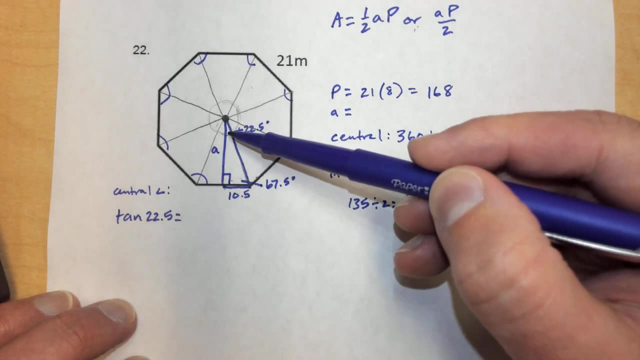 So we can use the tangent function with our 22.5 degree angle. So the 22.5, the tangent of 22.5, is going to be equal to the ratio of the opposite leg, which is 10.5,. 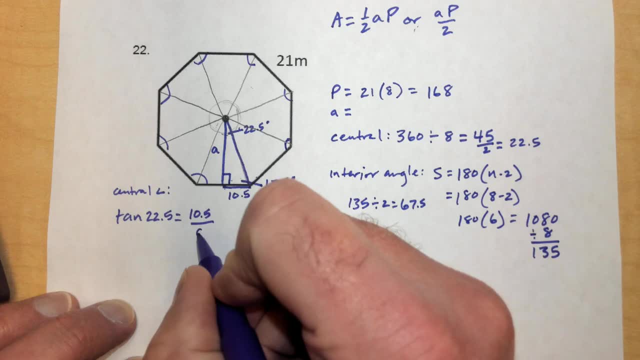 over the adjacent leg to the angle, which is the apothem we're looking for. And now we can do some cross multiplication and figure this out. I'm going to put it over 1, just so we can cross multiply. We get a times our apothem. 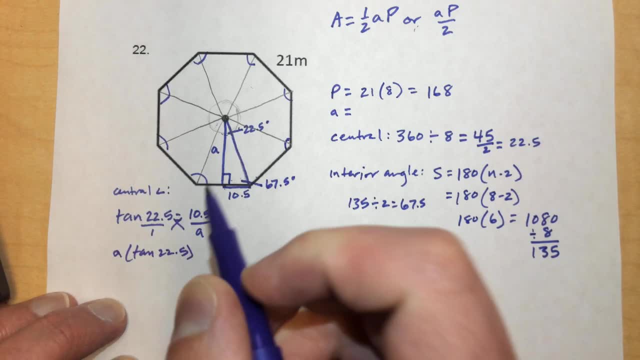 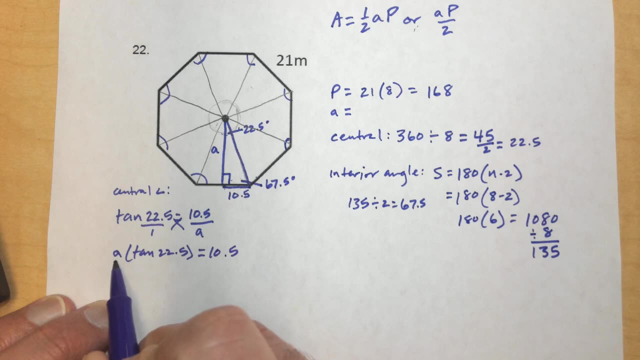 Times the tangent of 22.5.. That's going to be equal to 10.5 times 1,, which is 10.5.. And because we're trying to solve for the apothem, remember this tangent of 22 at 5 is just a decimal. 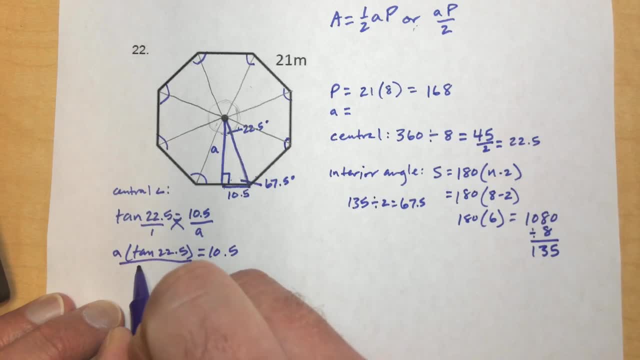 Okay, It's a never-ending decimal. We're going to divide by that decimal, which is the tangent of 22.5.. That way we can get our apothem by itself And because we're dividing here, we ultimately are going to be taking 10.5.. 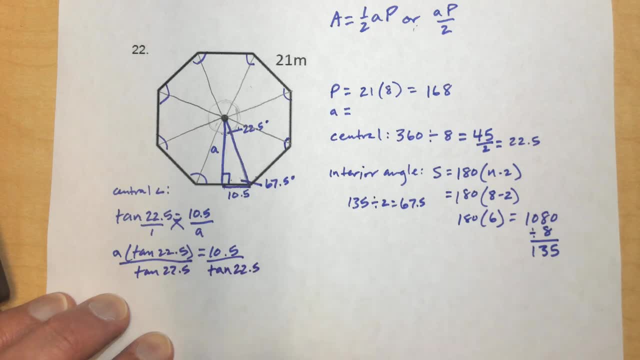 And dividing by the tangent of 22.5.. And when we do that, our apothem then is 25.35.. Now, just to show you that it'll work in this other angle, if you decided to do that and use the formula. 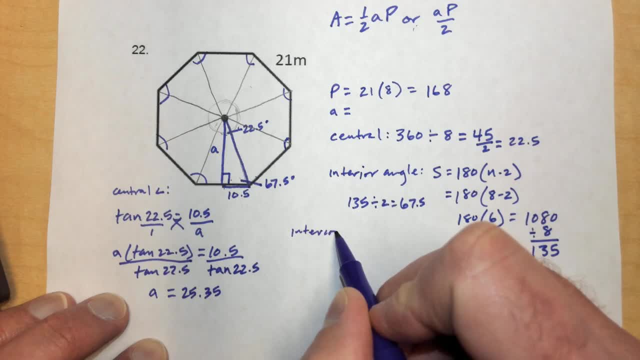 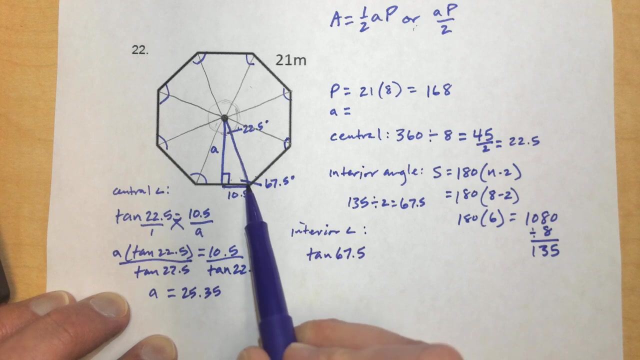 if we're using the interior angle- interior angle- we're still going to be using tangent. We're just going to be using the tangent of the 67.5 degree angle, Because the tangent of the 67.5 degree angle, if we use this ratio, that's going to be the opposite leg here. 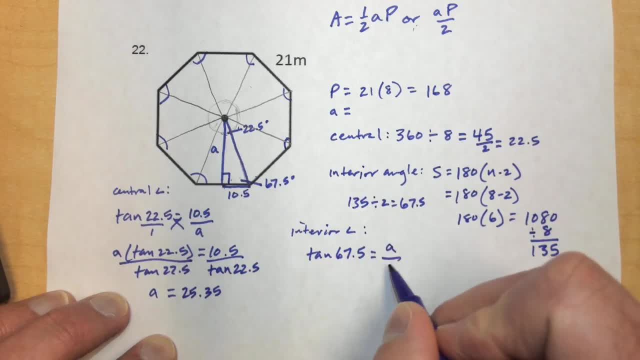 which is our apothem, over the adjacent leg, which is 10.5.. Notice in our ratios here, when we're using the opposite angle, the tangent ratio gets flipped. So we're using one angle. The apothem was on the bottom of the 10.5.. 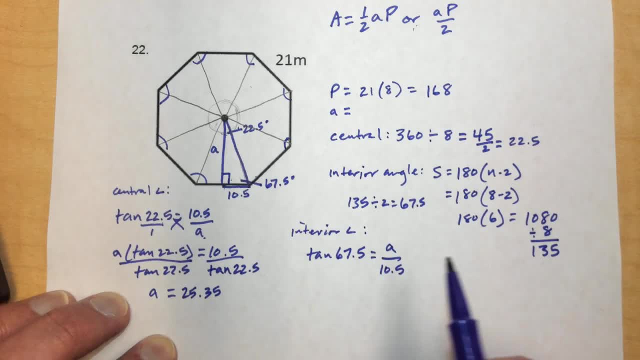 If we use the other angle, the apothem's on the top of the 10.5.. Okay, So when we put that over 1 and cross-multiply now we get A. our apothem is equal to 10.5 times the tangent of 67.5.. 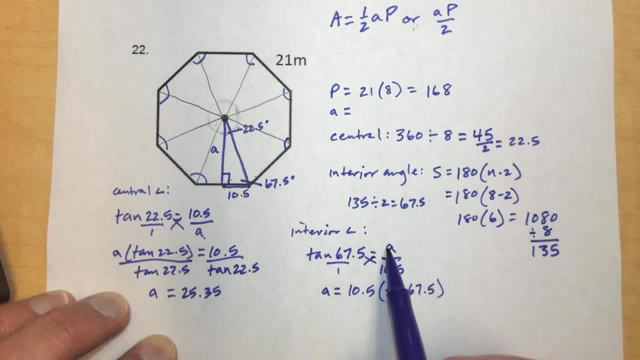 We were dividing over here because the apothem was on the bottom. Now, because the apothem is on the top of our ratio, we end up multiplying And if we multiply that out, we still get the apothem of 25.35.. 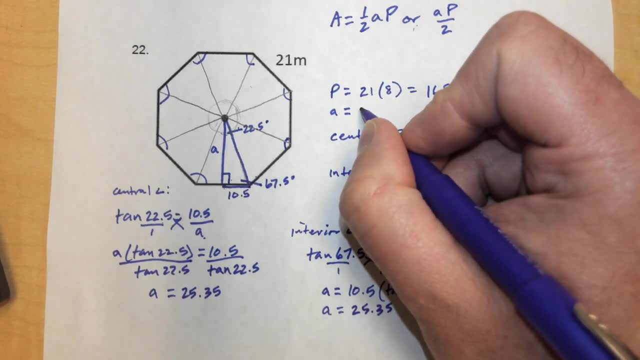 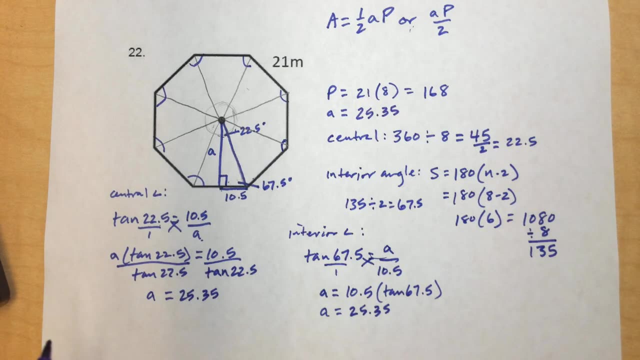 So we're going to go back up to the top here, And now that we've got our ratio, we're going to go back up to the top here, And now that we've got our apothem of 25.35, now all we have to do is plug that into our formula. 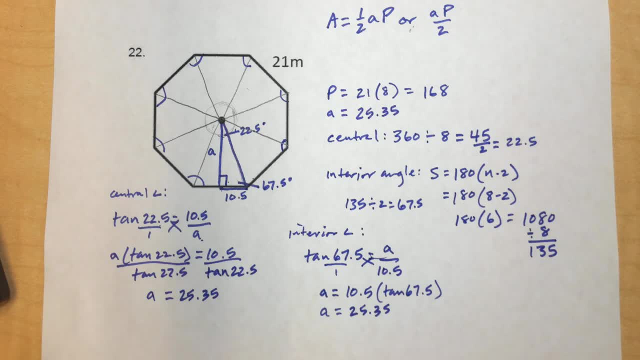 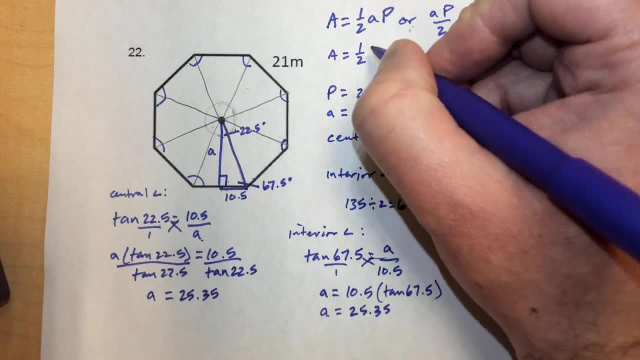 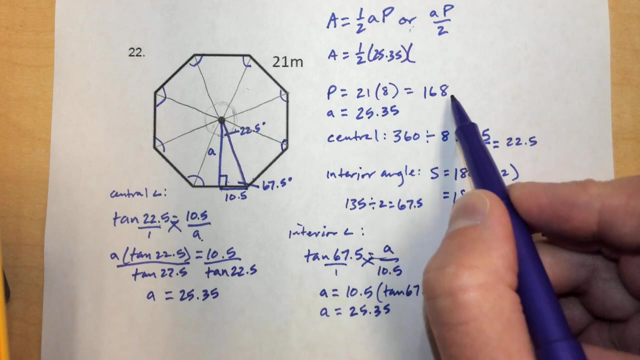 So we're going to take the 22.35 apothem. So our formula again is: the area is 1 half of the apothem, 25.35, times our perimeter, which we figured out earlier, which is 168.. 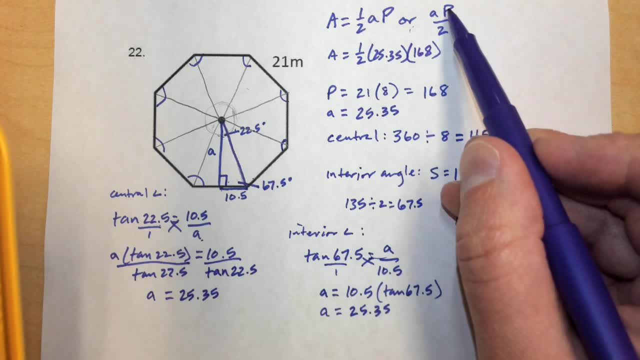 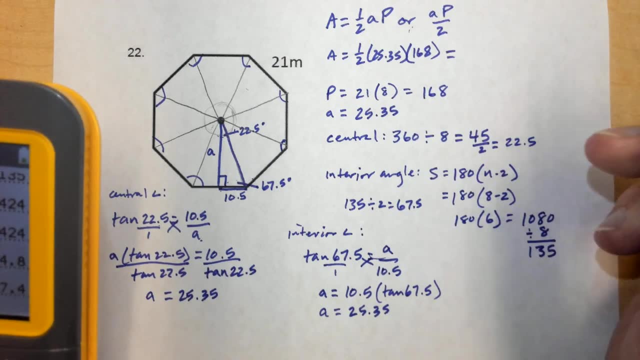 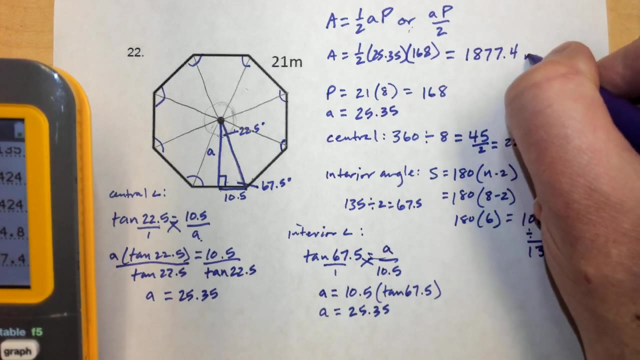 Okay, Again, that's the same as 168, the perimeter times the apothem divided by 2.. So you can plug it into that formula if you'd like as well. And if we multiply all that out, our answer should be 1,877.4 square meters. 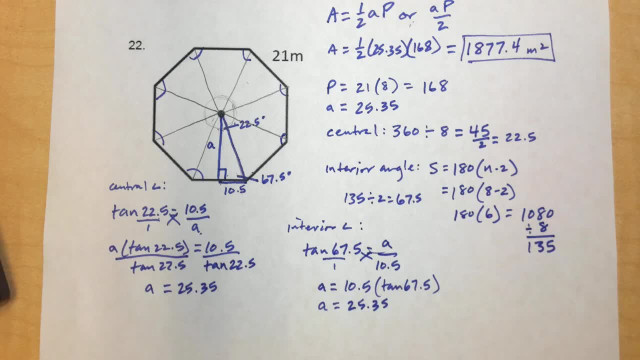 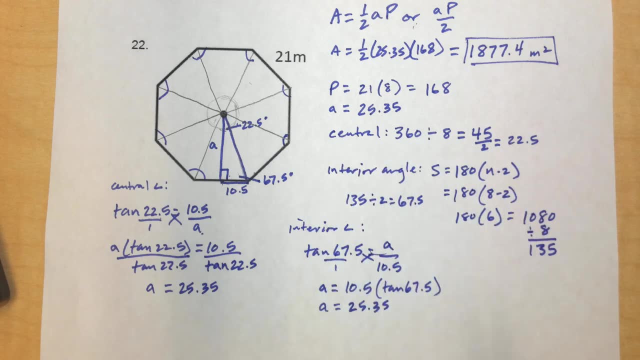 And there you have it. Yes, it was a lot of work, But again your work is going to look like about half of this, because you're going to choose either the central angle or the apothem Or the interior angle version to find one of these two angles. 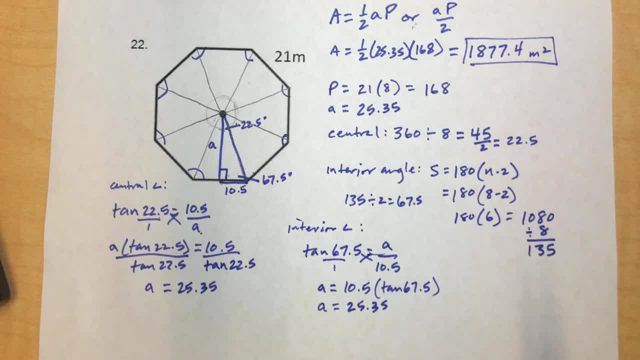 And then you're going to pick one of these formulas to use for finding the angle.